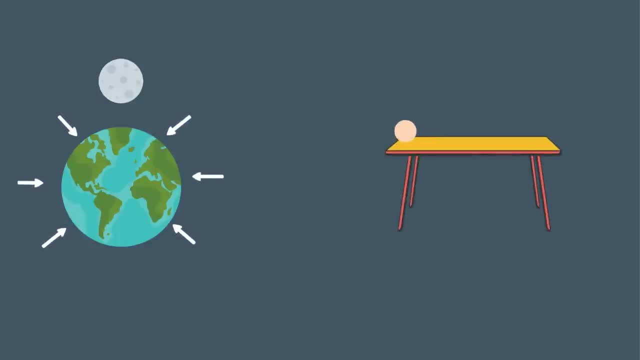 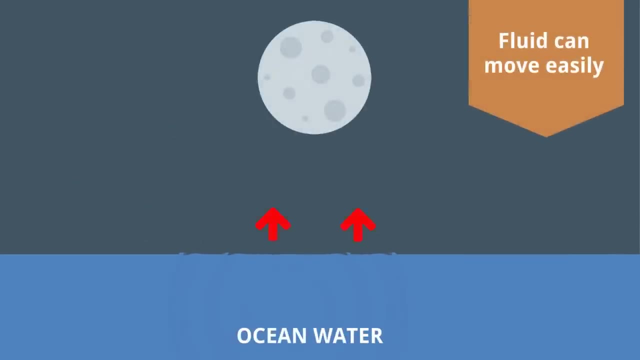 earth are grounded, Like if you throw a ball, it will fall due to the earth's gravitational pull, But the ocean water being fluid which can able to flow easily, it can be pulled towards the moon and this is what creates the tide. 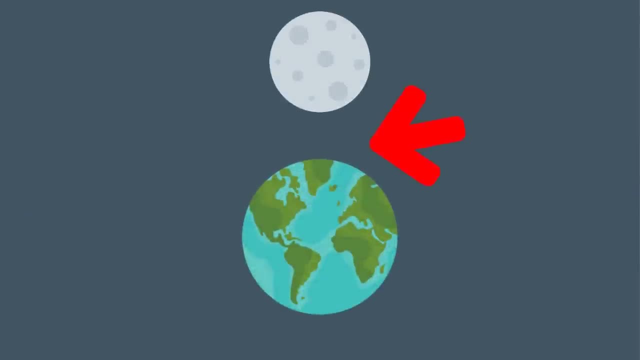 So the side of the earth closest to the moon experience the strong gravitational pull of the moon, which causes the sea to rise, creating high tides. High tide will form on the other side too. This happens because this side is further away from the moon and the 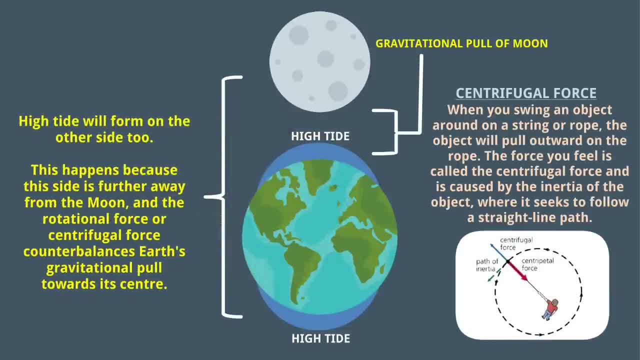 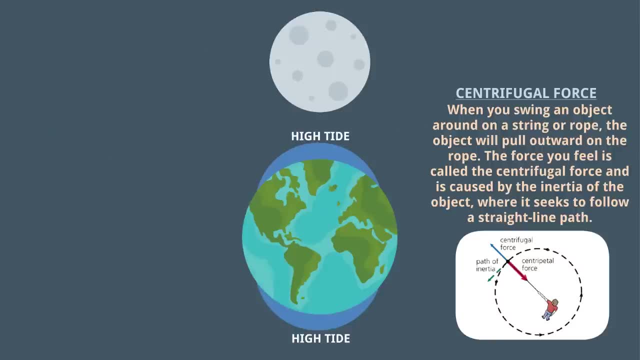 centrifugal force counter-balances earth's gravitational pull towards its center. So there are two tidal rises created on the opposite sides of the earth, and they are earth. one is due to the gravitational pull of the moon and the other is due to the centrifugal force. 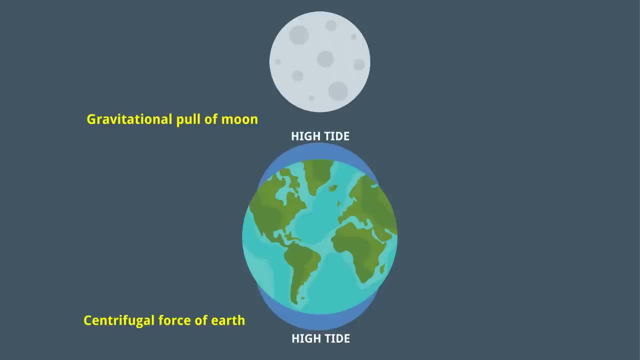 of the earth. since ocean water is pulled higher in the areas of the two high tides, there is less water in between two high tides. these areas are the low tide areas. the high tides and low tides occur only when there is moon and the earth. so what is the role of sun in the tide? sun is the 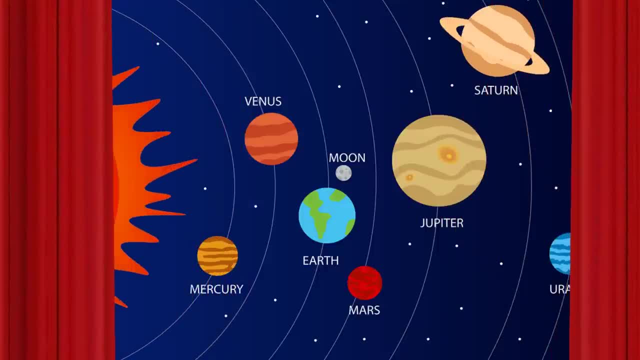 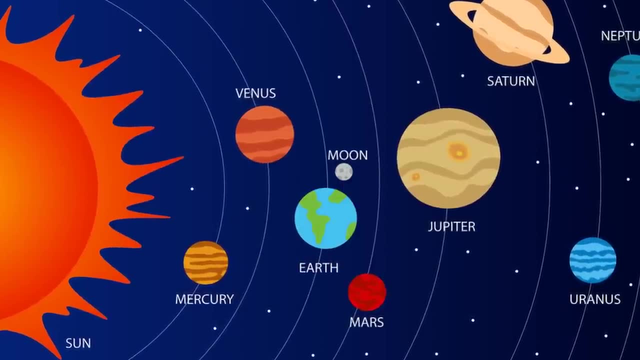 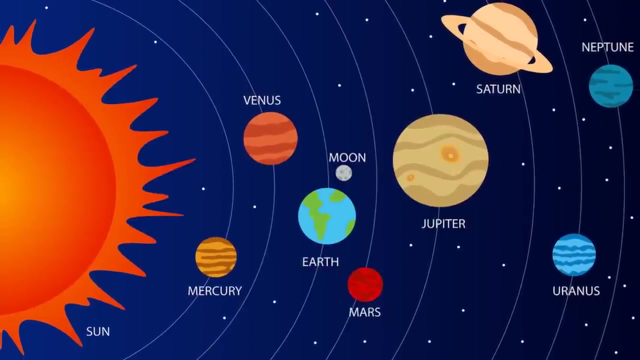 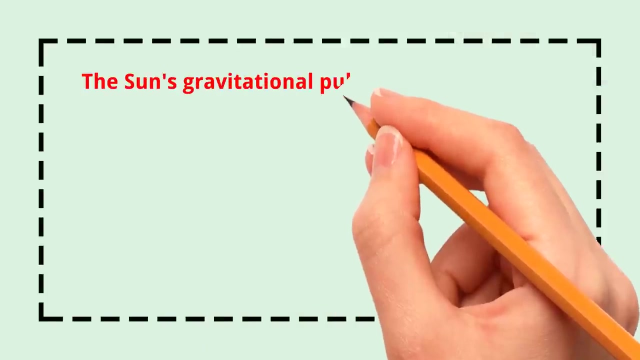 most significant celestial body in our solar system. its gravity holds the solar system together, keeping everything from the biggest planet to the smallest particle of debris in its orbit. that means the sun exert more gravitational pull and it has an influence on the tides as well. however, the sun's gravitational pull can do two things either. it will increase the moon's 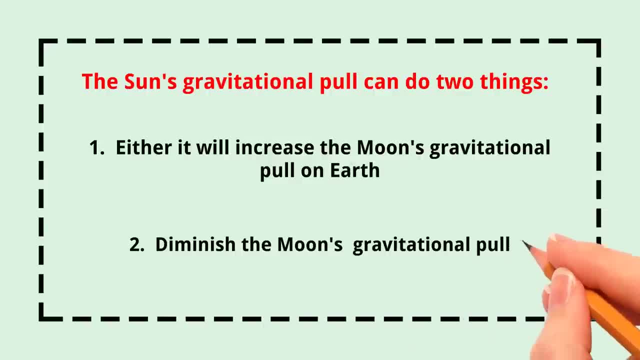 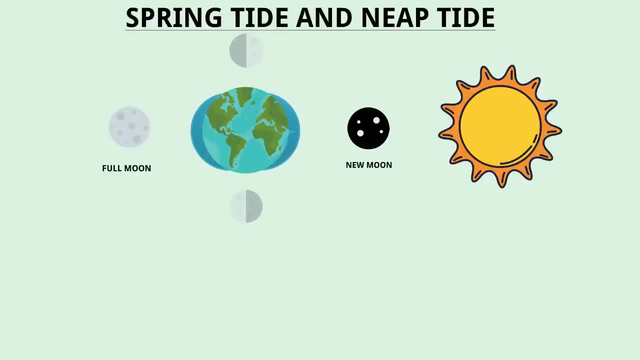 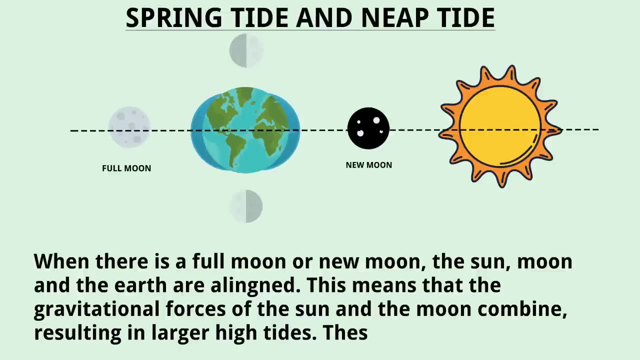 gravitational pull on the earth or diminish the gravitational pull on earth. during the full moon and new moon phases, the sun, earth and moon arrange themselves more or less along a line in space. then the pull on the tides increases because the gravity of the sun reinforces the moon's gravity. thus in a new moon or a full moon, 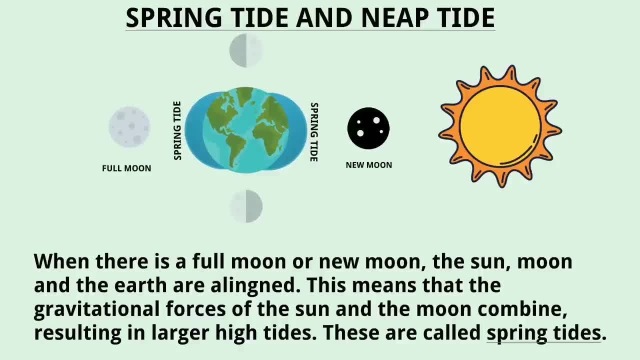 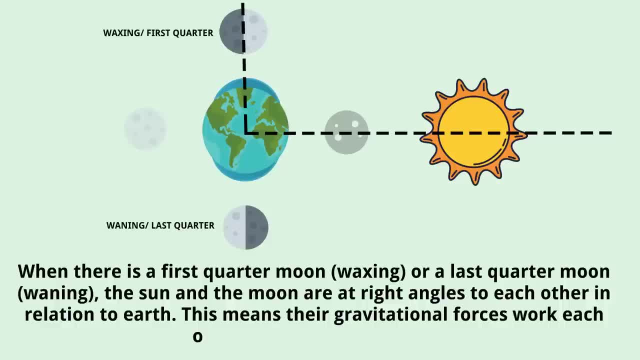 the tide range is at maximum. this is spring tide and during waxing and waning moons the Sun and the moon are at right angles as seen from Earth, Then Sun's gravity is working against the gravity of the moon as the moon pulls on the sea.